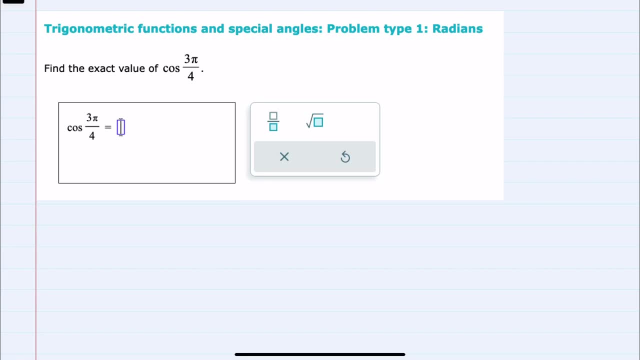 In this video I'll be helping you with the Alex problem type called Trigonometric Functions and Special Angles. Problem Type 1, Radians. We're asked here to find the exact value of cosine 3, pi, fourths and for any of the special angles. I like to think back to our unit circle. 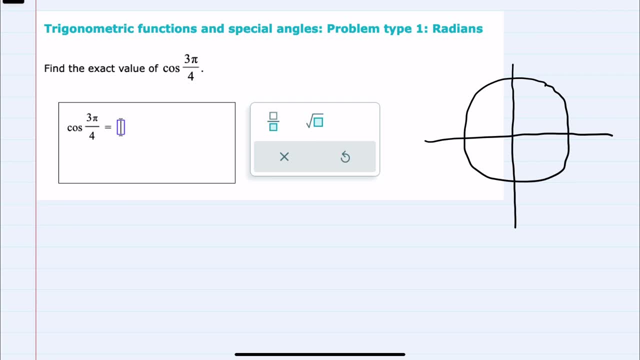 put in all the special angles and their values for quadrant 1, and then use quadrant 1 to find any of the special angles that fall into other quadrants. So I'll start by labeling our axes here in radians as 0 radians. pi is halfway around the circle, so pi halves is in the middle. 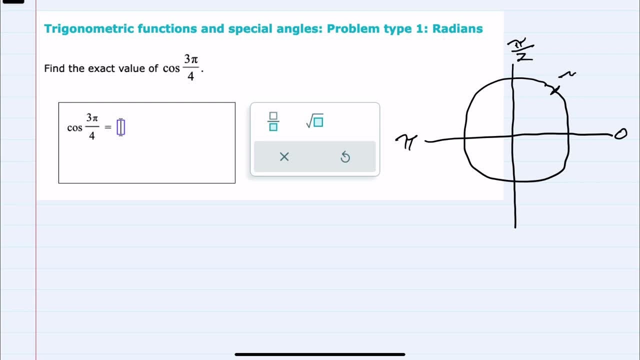 and then the multiples of pi fourths, As well as the multiples of pi sixths, which includes 2 pi sixths, which is pi thirds. So these are all of our special angles in quadrant 1, and the values starting at 0,. 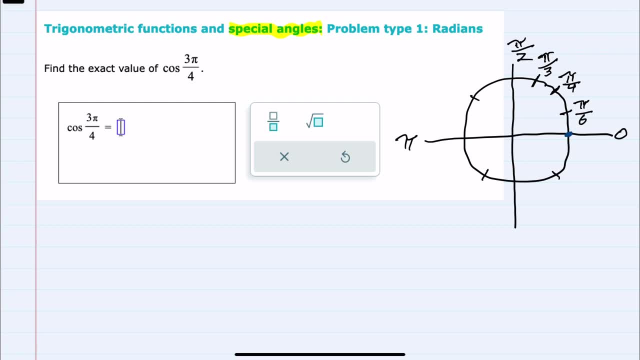 so one unit is our x value, so this would be 1, 0.. And then, as we've discussed in other videos, this is a unit circle, so one unit is our x value, so this would be 1, 0. 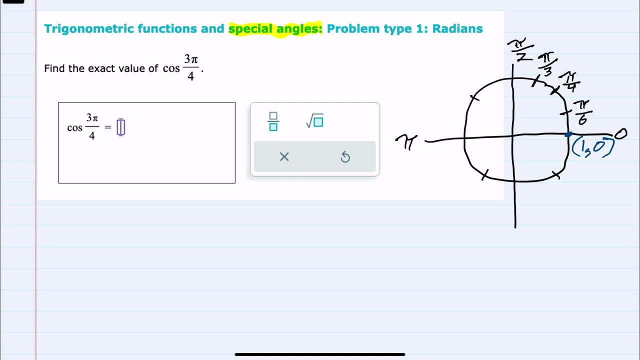 and then, as we've discussed in other videos, this would be 1, 0.. The pattern is about square roots over 2.. So thinking of 1 as the square root of 4 over 2, next would be the square root of 3 over 2,. 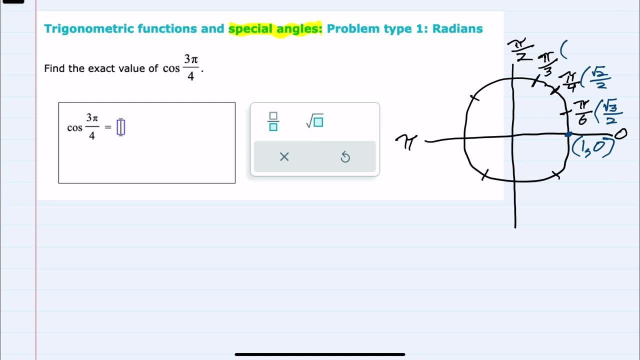 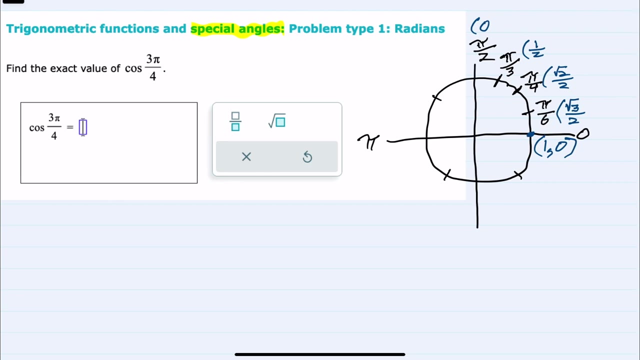 then the square root of 2 over 2, then the square root of 1 over 2 is just 1 half and the square root of 0 over 2 is 0.. Following the opposite pattern for our y values, we started with 0, which was the square root of 0 over 2,. 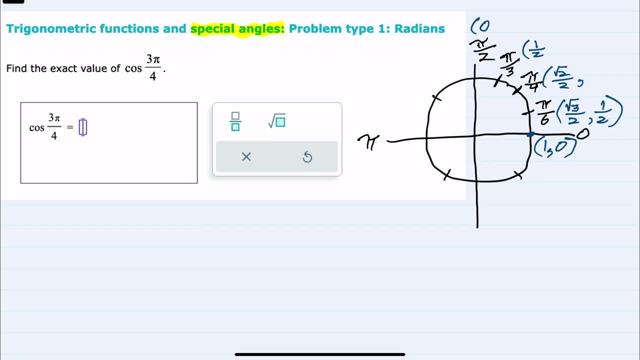 then the square root of 1 over 2 is 1, half the square root of 2 over 2, the square root of 3 over 2, and then the square root of 4 over 2 is just 1.. 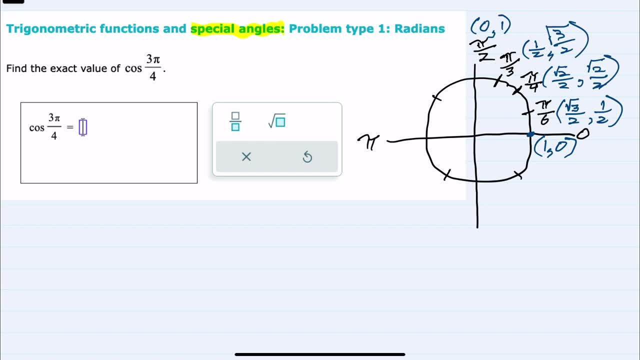 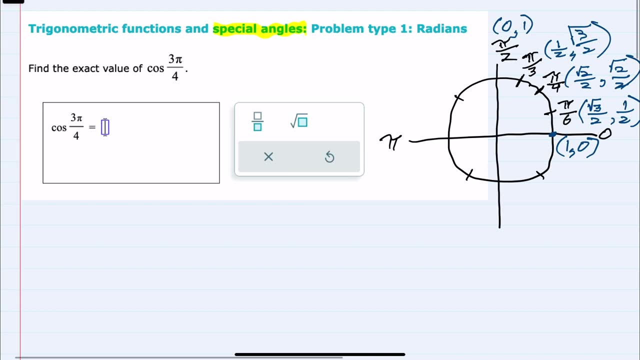 So at this point we have all of our special angle cosine and sine values, our x's and y's here in blue, And I can look back and I see that for this question we're looking at 3 pi 4.. So this is a multiple of pi 4s.